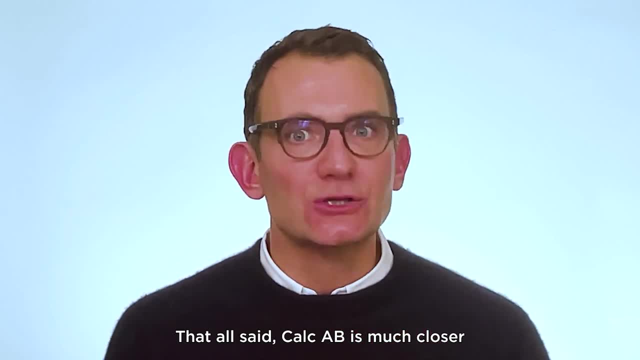 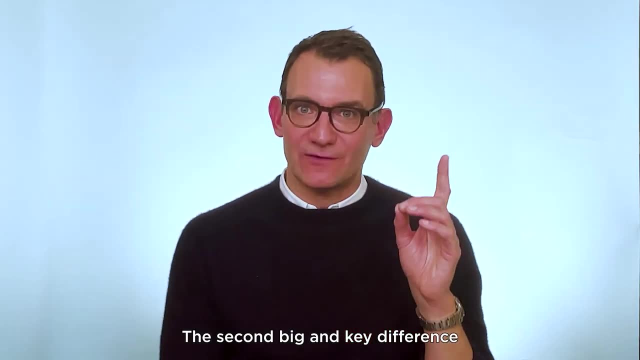 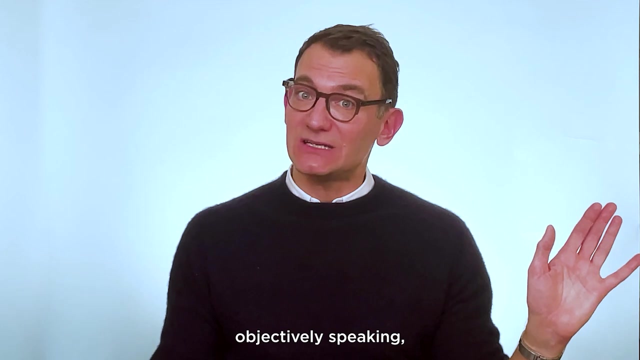 That all said, calc AB is much closer to covering three-quarters of a year of college-level calculus. The second big and key difference is that calculus BC covers more theoretical aspects of calculus and is, objectively speaking, much harder than calculus AB. Now the AB exam. 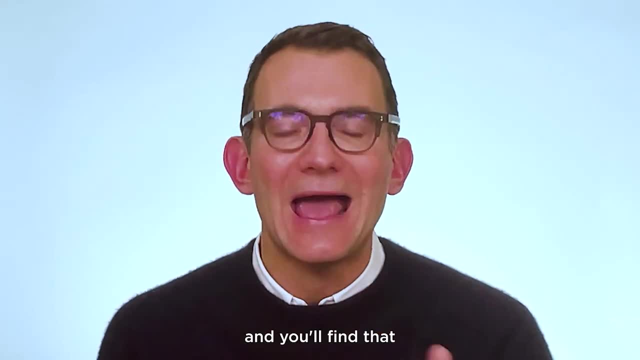 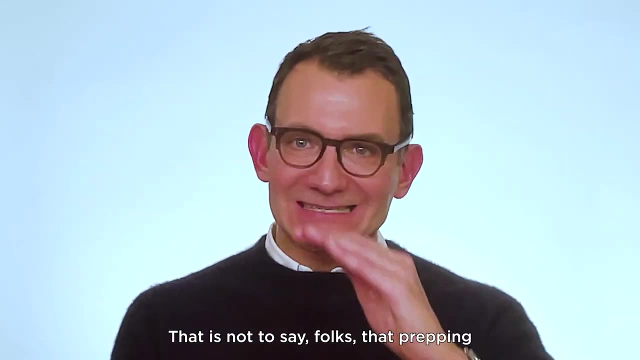 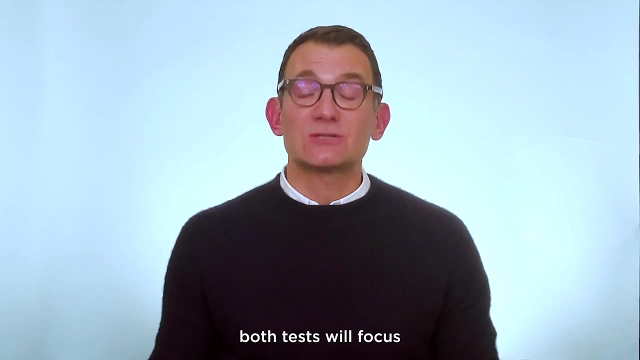 usually tests more straightforward problems and you'll find that the problems aren't as tricky or as varied as the problems that you'll find in the BC exam. That is not to say, folks, that prepping for the AB exam will be super easy. Remember that both tests will focus on the basics. 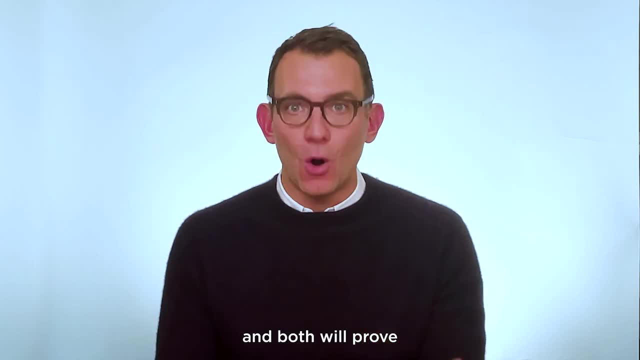 of differential and integral calculus, and both will prove to be difficult, mainly due to the breadth of the concepts that they cover. Now, the standard calculus AB exam is 3 hours and 15 minutes long, with a total of 51 questions. Those 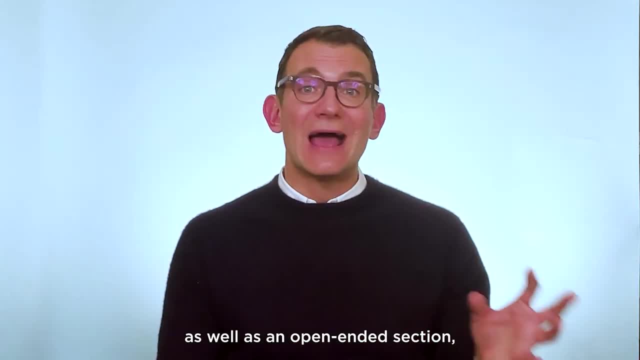 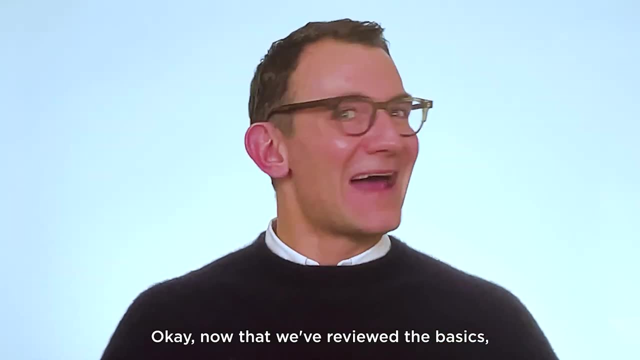 questions are divided into two sections, with a multiple-choice section as well as an open-ended section. Both sections will include a calculator and a non-calculator portion. Okay, now that we've reviewed the basics, we should tackle the key concepts that you'll need. 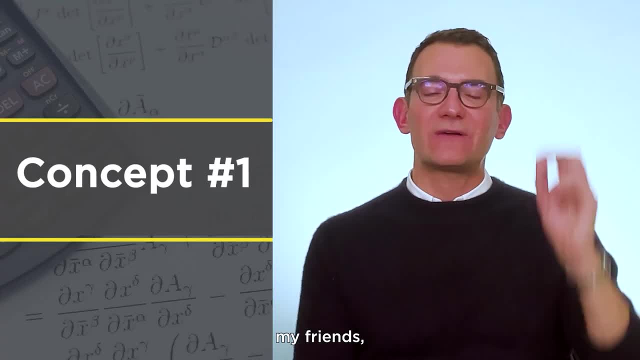 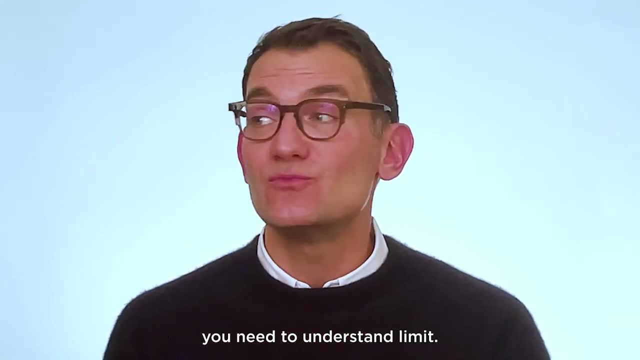 to have at the ready come exam day. Concept number one, my friends—limits, asymptotes and continuity. Now, in order to understand calculus functions, you need to understand limits. Limits are the foundation of important definitions and theorems that will be. 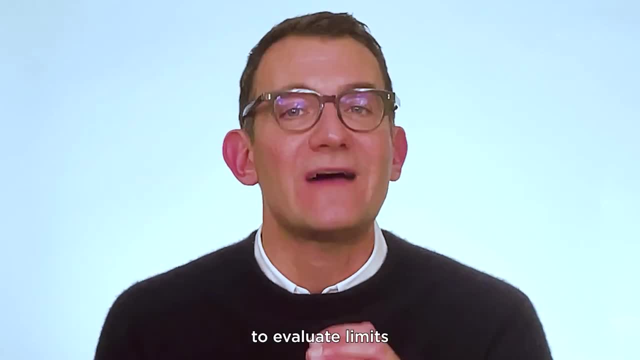 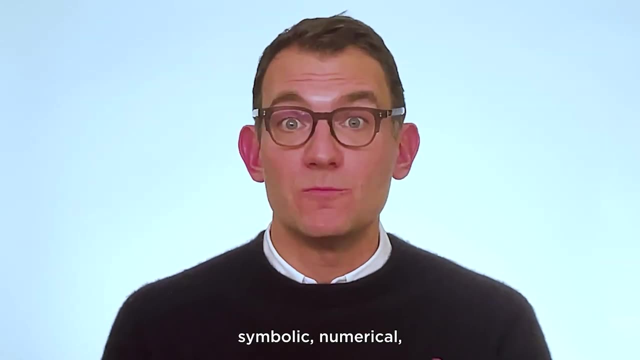 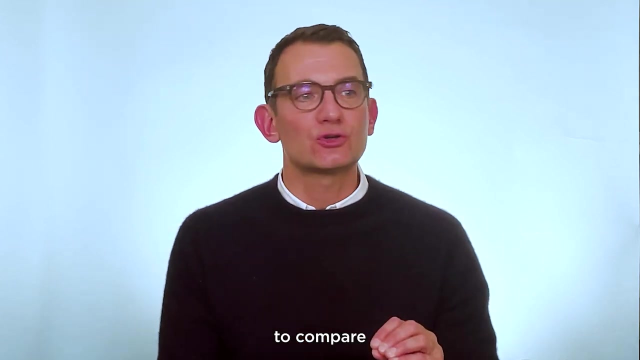 tested throughout the degree. Aim to evaluate limits not only from equations, but also graphically, symbolically, numerically and also by any basic or formal method. You should understand asymptotes graphically and be sure to be able to consistingly compare its growth rates. 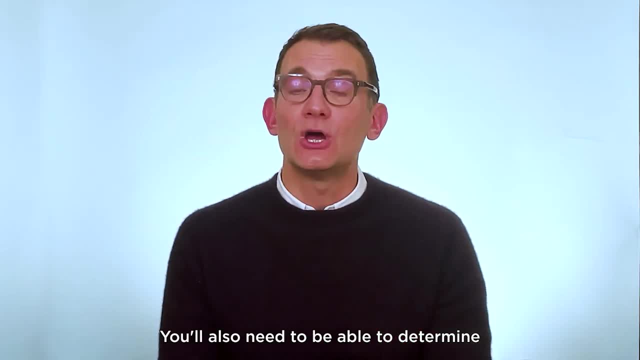 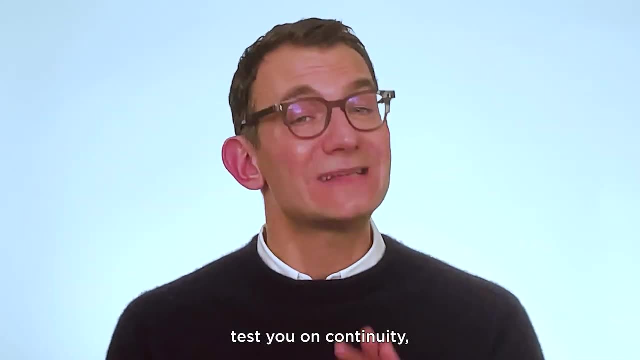 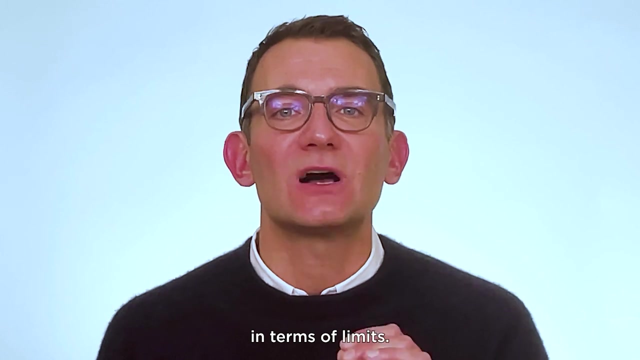 different types of functions. you'll also need to be able to determine asymptotes and limits at infinity. now, the ap exam will also test you on continuity, so you should be able to test the continuity of a function in terms of limits, and you should understand continuous functions. 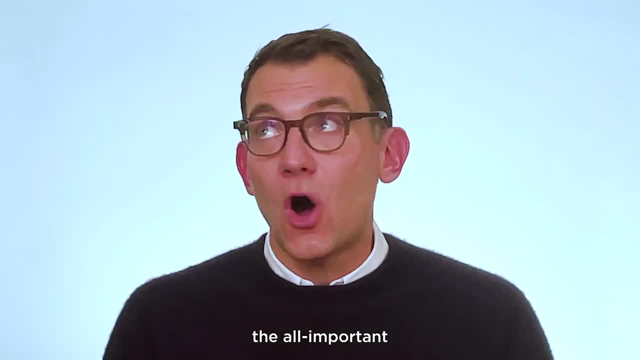 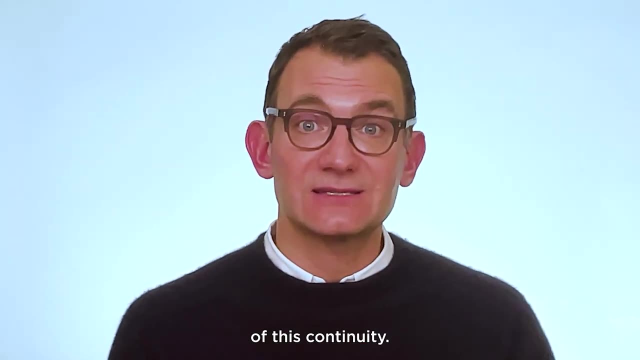 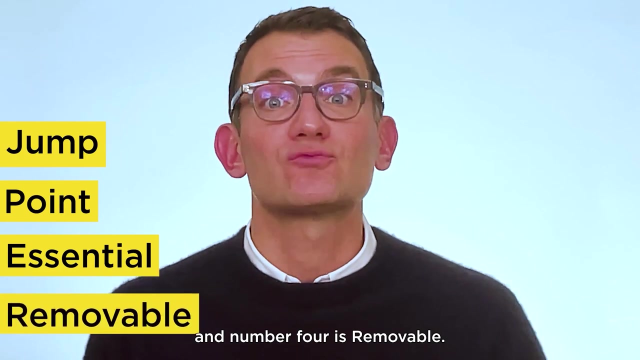 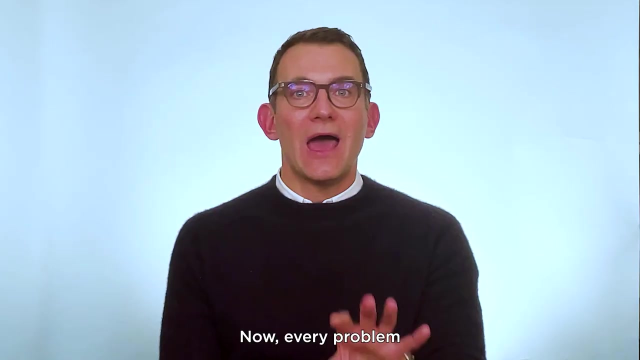 graphically. now you should also understand the all-important intermediate value theorem, as well as the four different types of this, uh, uh, continuities. now the first one, jump. second point, third, essential. and number four is removable. that leads us on to concept number two, which is the definition of the derivative. now, every problem that you'll 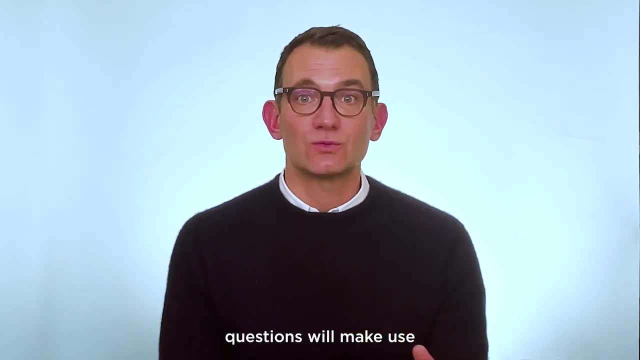 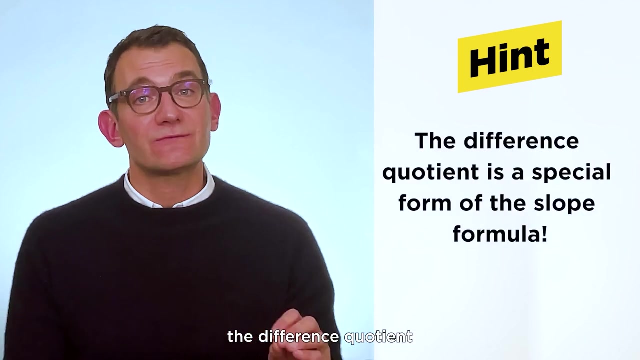 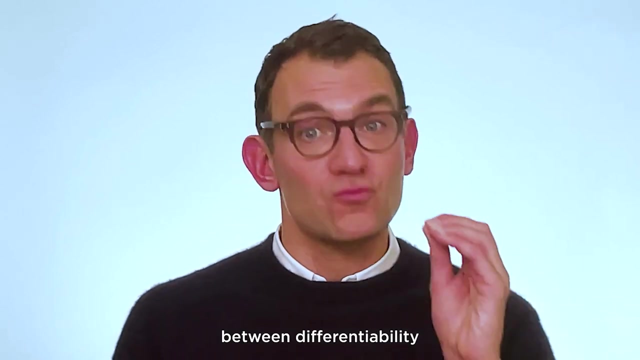 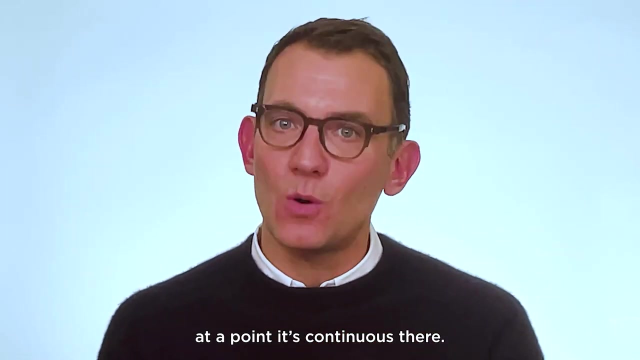 encounter on the differential calculus questions will make use of the derivative now, of course, hence the name. by test date you should be able to find a derivative by finding the limit of the difference quotient. You should also know the relationship between differentiability and continuity, That is, if a function is differentiable at a point, it is continuous there. 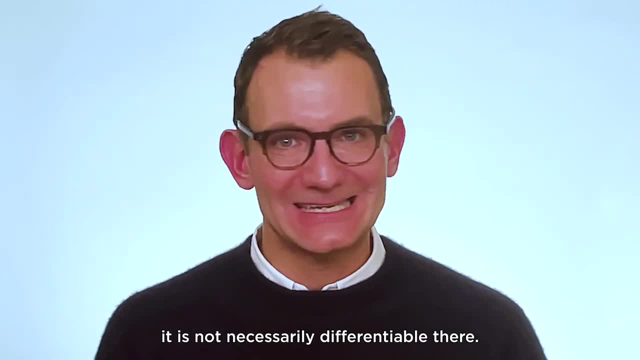 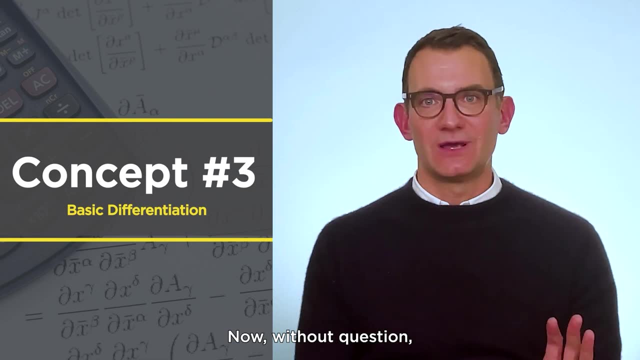 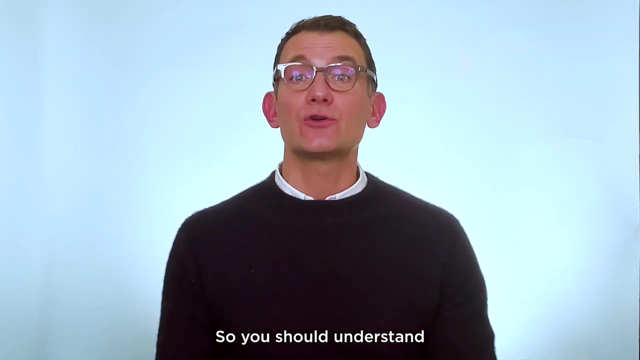 If a function is continuous at a point, it is not necessarily differentiable. there Leads me to concept number three, which is basic differentiation. Without question, the exam will test your mastery of the basic differentiation rule. You should understand the applications of the power rule, the product rule, the quotient. 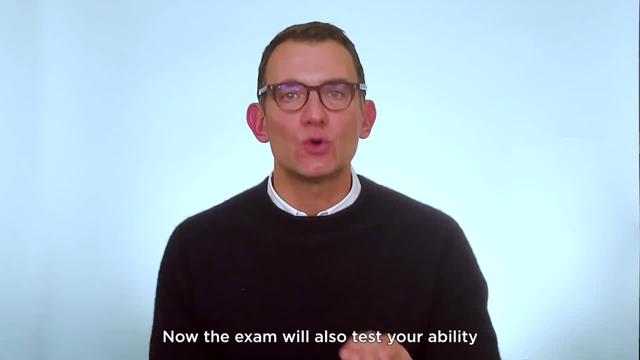 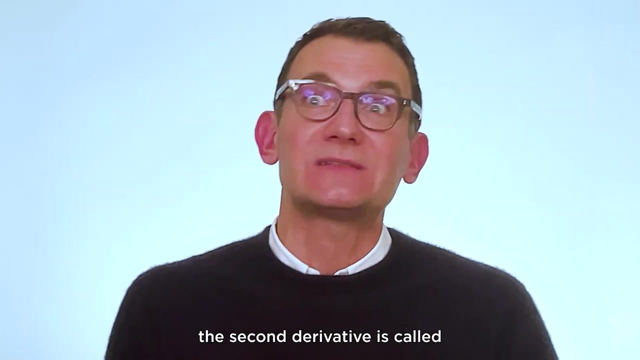 rule and the chain rule. The exam will also test your ability to find higher-order derivatives by taking the derivative of a function more than once. The derivative of the first derivative is called the second derivative, and the derivative of the second derivative is called the third derivative, and so on. 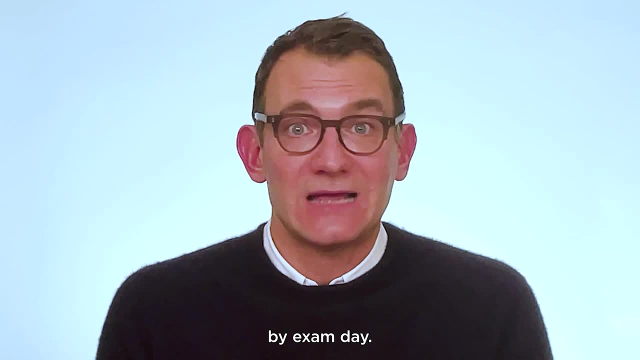 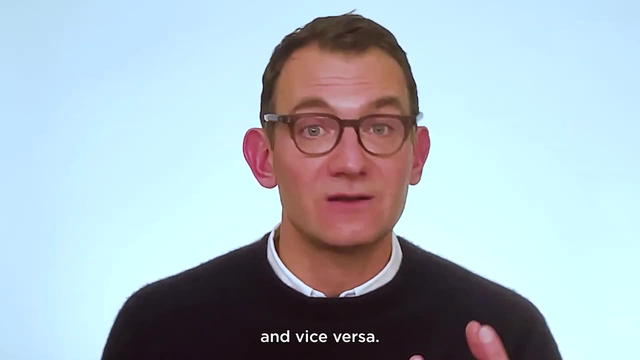 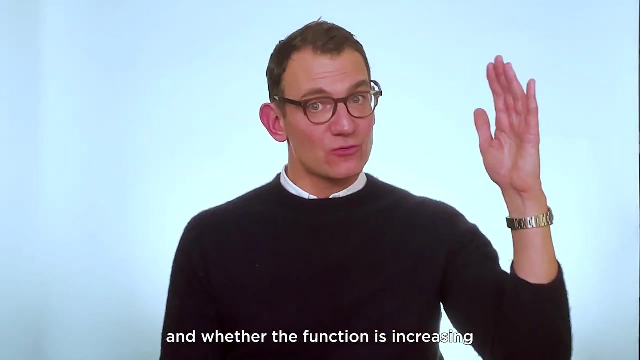 You should be clear on these concepts by exam days. You should also know how to relate the graph of a function to the graph of its derivative, and vice versa. Finally, you should understand the relationship between the sign of a derivative and whether the function is increasing or decreasing. 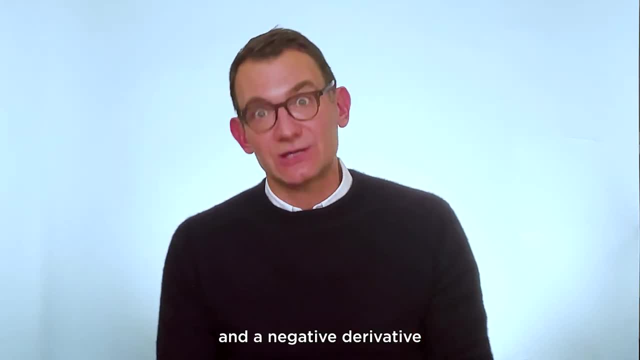 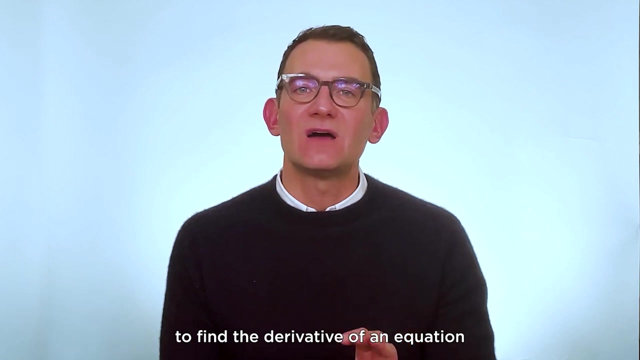 A positive derivative is increasing, A derivative is decreasing- increasing and a negative derivative means that it's decreasing. Concept number four, my friends, is implicit differentiation. You should expect to be tested on your ability to use implicit differentiation in cases when you're asked to find the derivative. 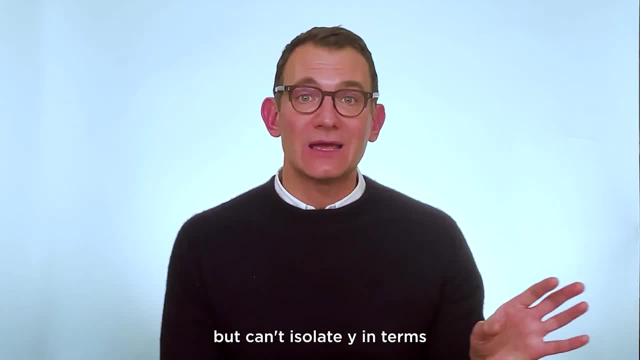 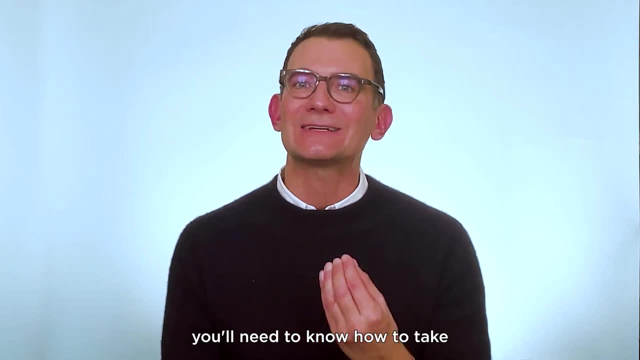 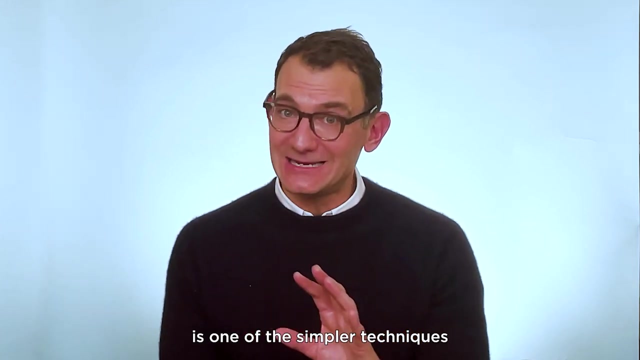 of an equation, but can't isolate y in terms of x, meaning that you can't differentiate this equation explicitly. You'll need to know how to take the derivative implicitly Now, while implicit differentiation is one of the simpler techniques you need to learn in calculus. 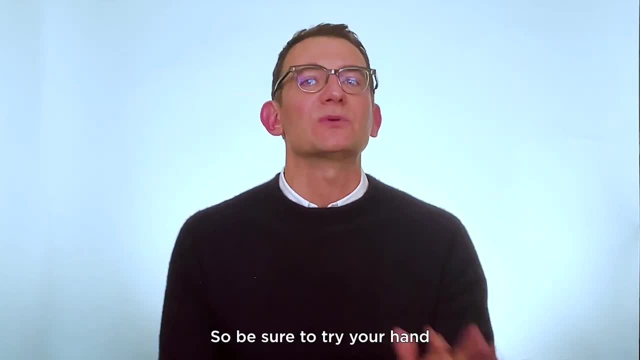 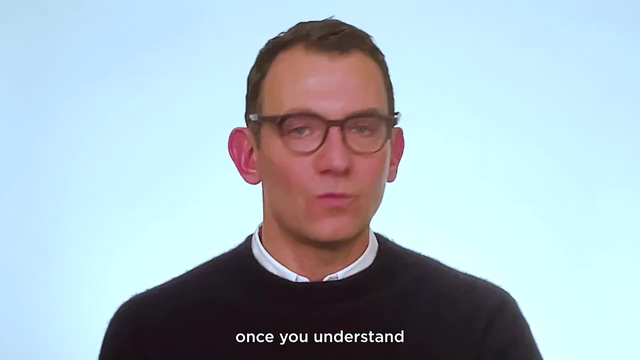 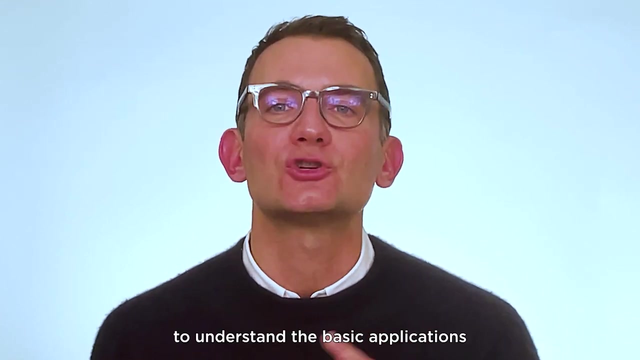 it can initially give many students trouble, so be sure to try your hand at plenty of practice problems. Concept number five is, of course, basic applications of the derivative. Now, once you understand the fundamentals of basic and implicit differentiation, it's important to understand the basic applications of the derivative. This includes: 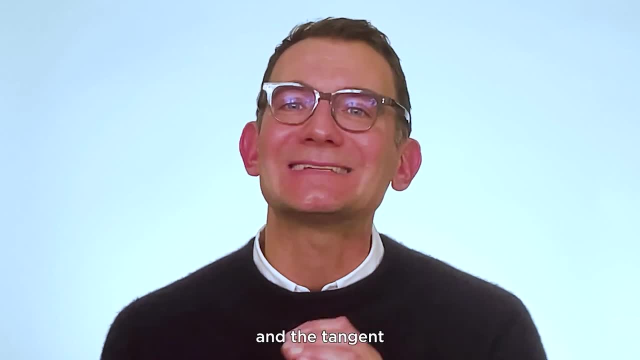 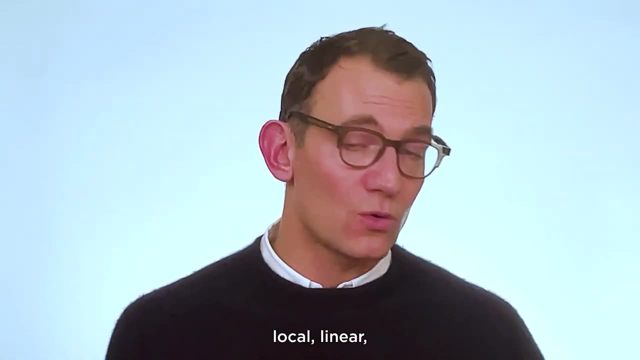 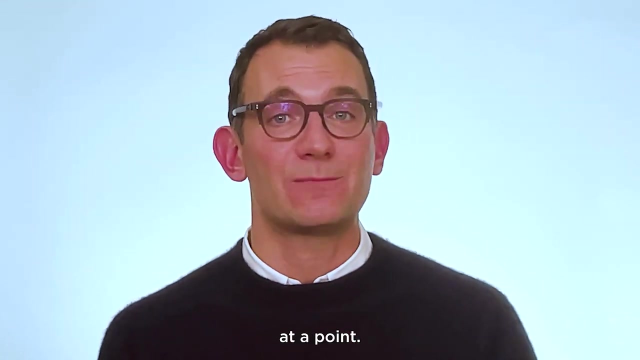 the ability to find the slope of a curve at a point and the tangent and normal lines of a curve at a point. This also means being able to use local linear approximation and differentials to estimate the tangent line to a curve at a point. You can also expect to see questions related to: 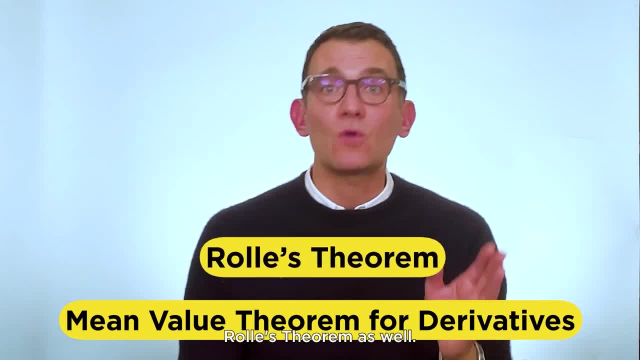 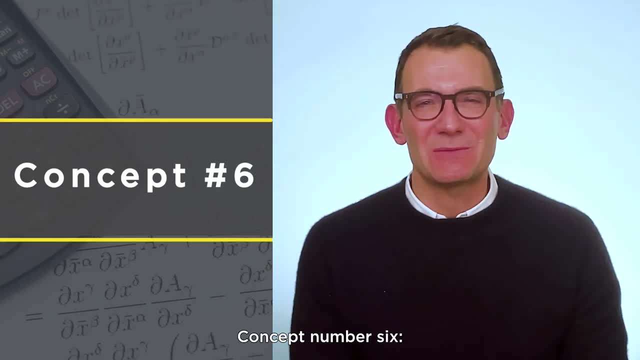 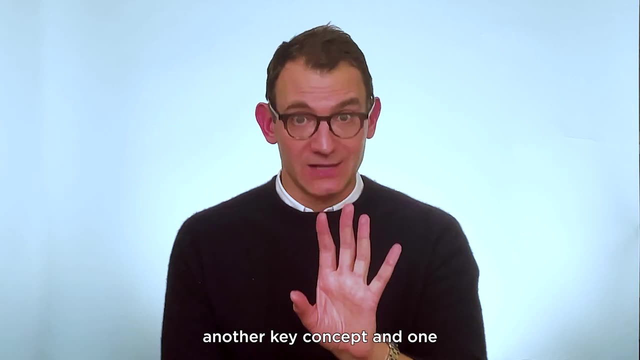 the derivative's value theorem and, of course, the Rolle's theorem. Be sure to review those applications in full and in detail before the exam. Concept number six is maxima minima and curve sketching Friends- another key concept—and one of the most common applications. 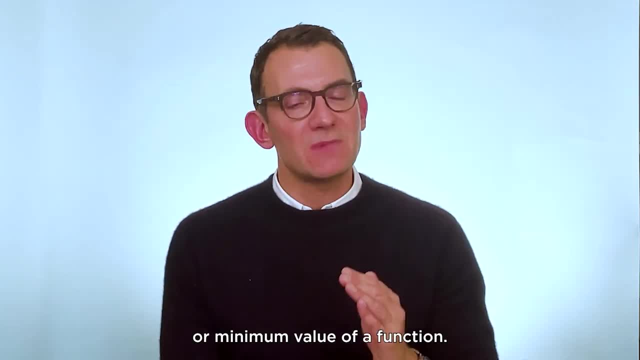 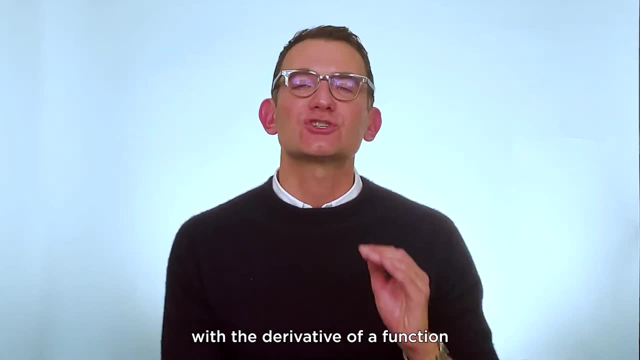 of the derivative—is to find the maximum or minimum value of a function. The maximum or minimum value of a function occurs at a point and the maximum value of a function occurs at a point where the derivative of a function is zero. These values can be called extreme values. 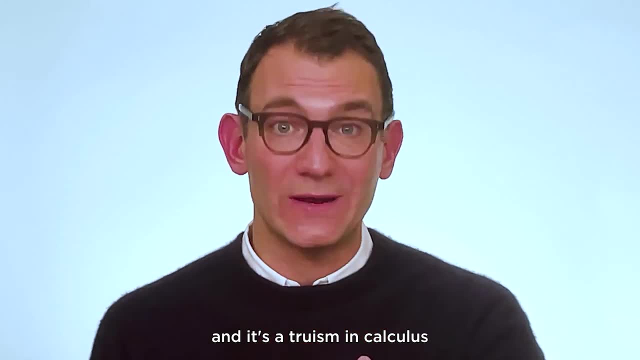 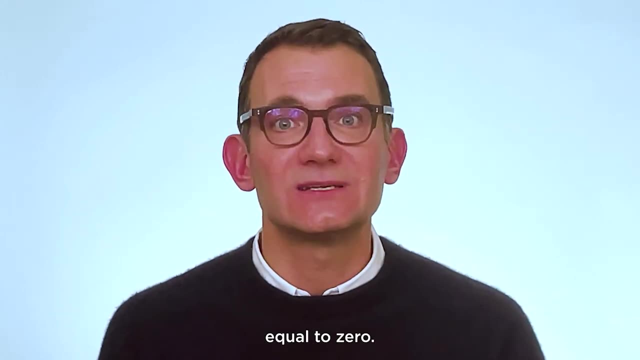 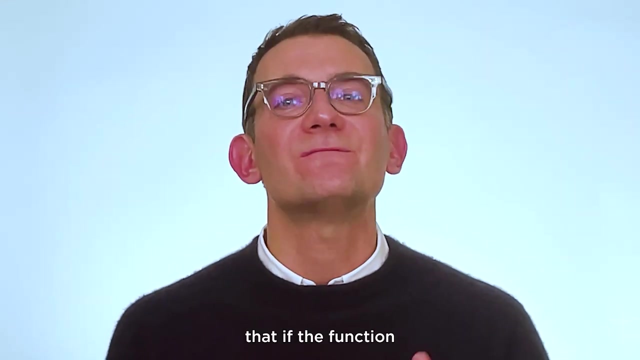 optimal values or, of course, critical points. It's a truism in calculus that if you don't know what to do, take the derivative and set it equal to zero. You should also be familiar with the extreme value theorem, which explains that if the function is continuous in an interval, 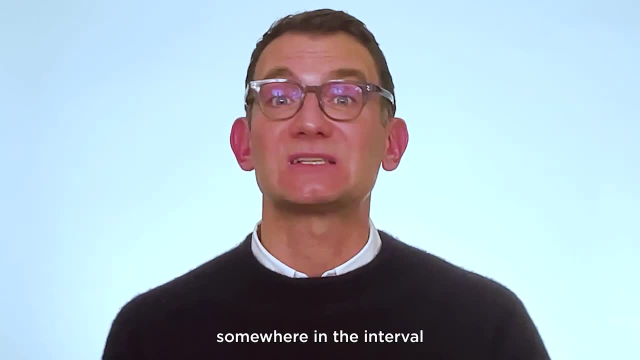 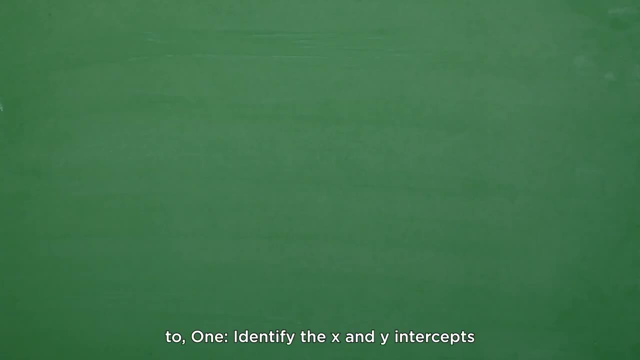 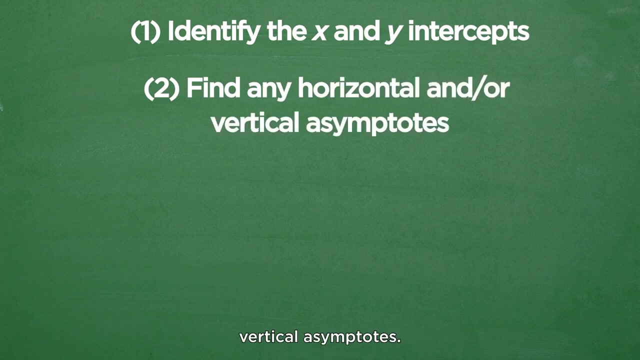 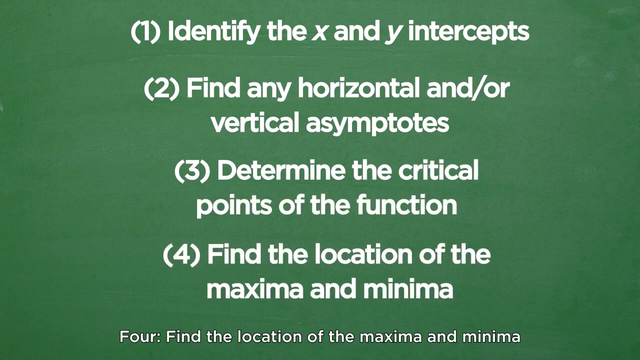 then you must always have a maximum or a minimum somewhere. You should also know how to sketch a curve. This means being able to identify the x and y intercepts, find any horizontal and or vertical asymptotes, determine the critical points of a function, find the location of the maxima and minima and determine the points of inflection. 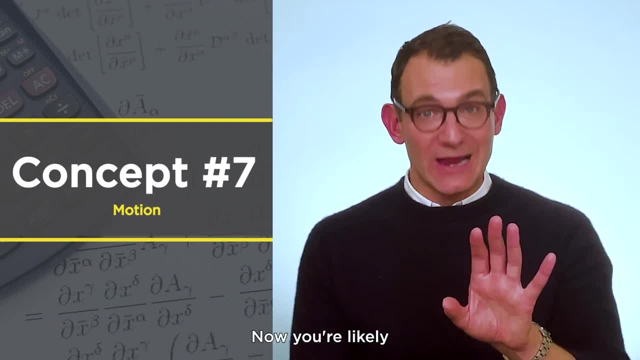 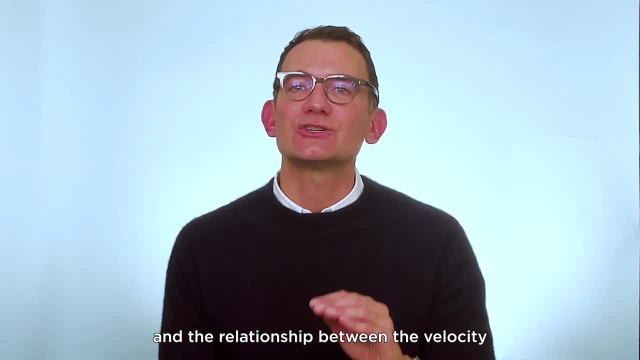 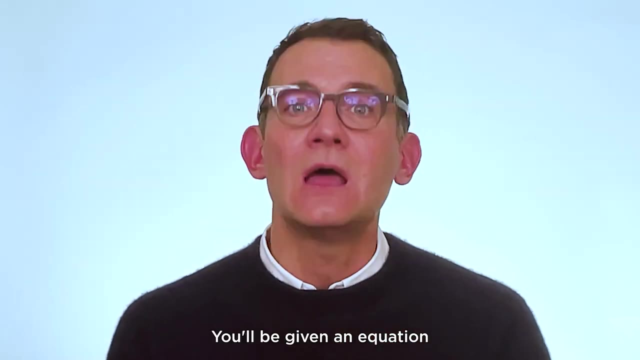 That brings us to concept number seven, which is motion. Now you're likely to see some basic problems about motion on the exam, specifically unrelated rates and the relationship between the velocity and acceleration of a particle. For related rate problems, the idea is pretty simple: You'll be given an equation relating to two or more variables. 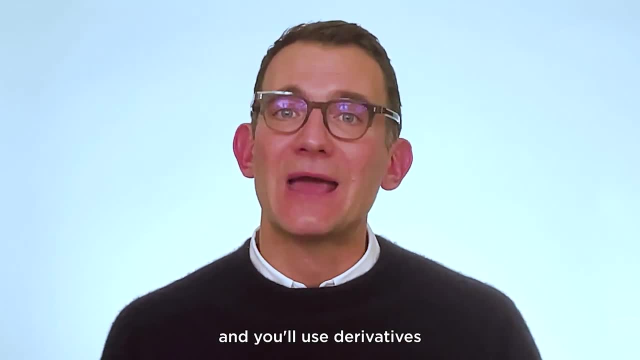 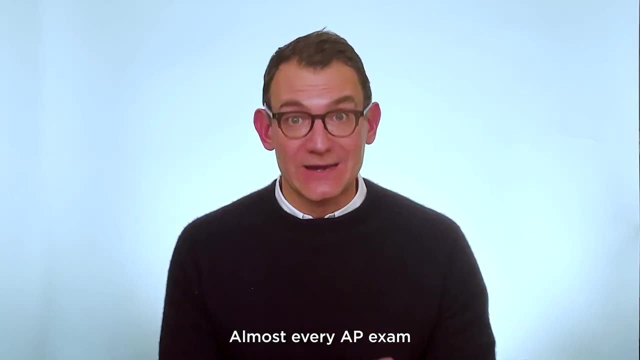 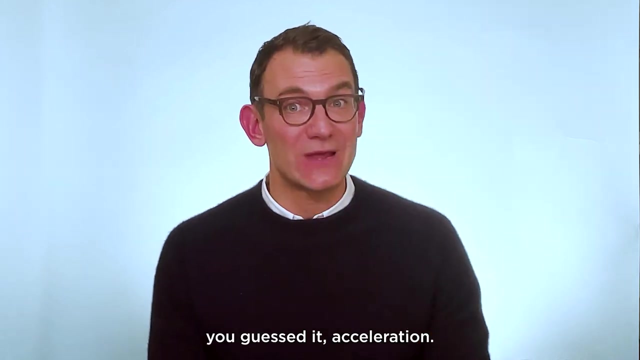 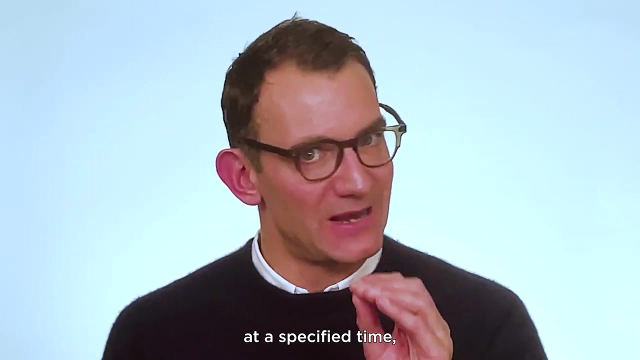 These variables will change with respect to time and you'll use derivatives to determine how the rates of change are related. Almost every AP exam will also have a question on position, velocity and acceleration. If you have a function that gives you the position of an object, usually called a particle, at a specified time. 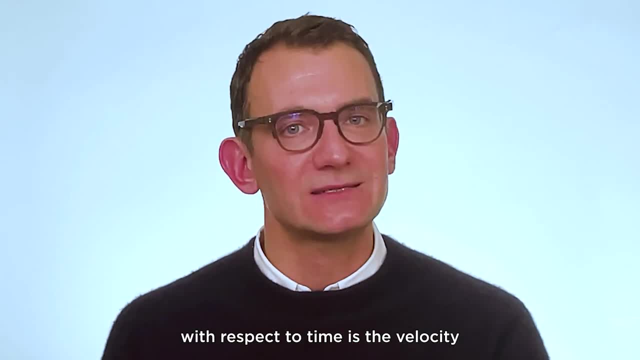 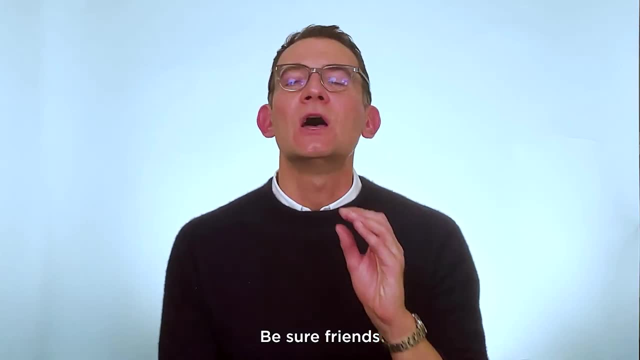 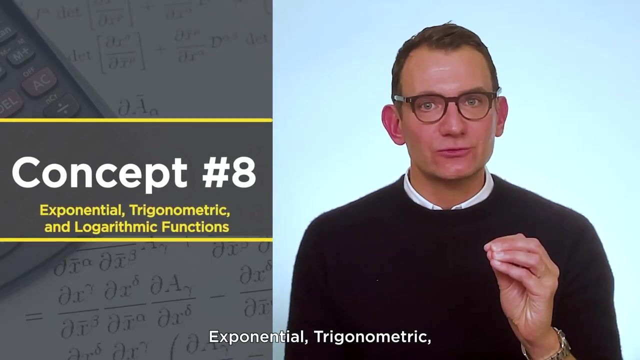 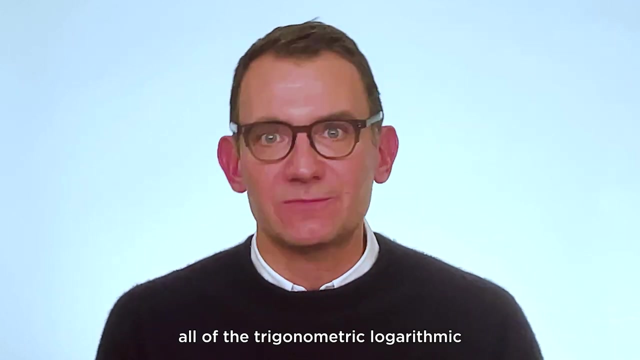 then the derivative of that function with respect to time is the velocity of the object and the second derivative is the acceleration. Be sure to familiarize yourself with these concepts by testing them. Concept number eight: exponential, trigonometric and logarithmic functions. Remember all of the trigonometric, logarithmic and exponential functions. 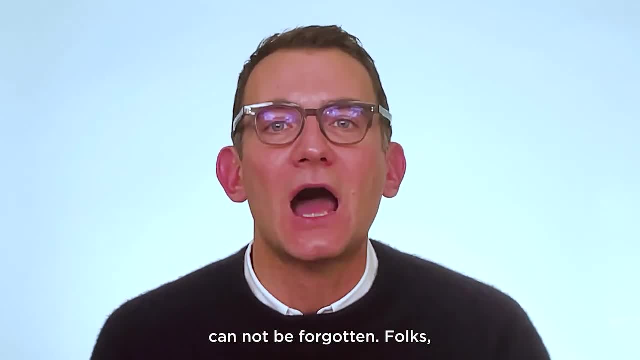 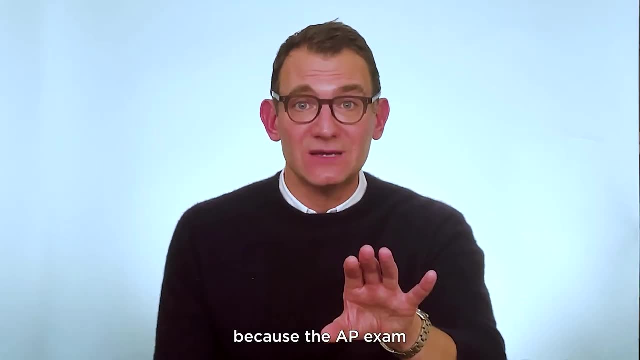 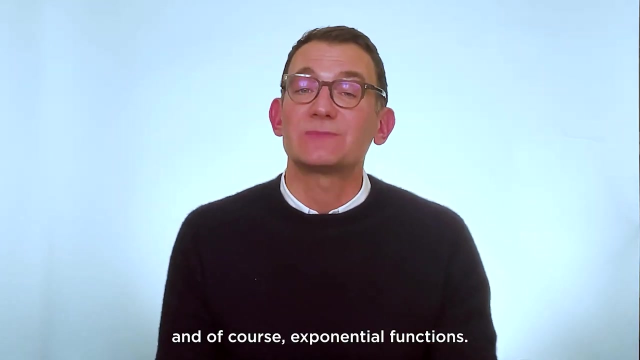 that you studied in pre-calculus cannot be forgotten. That said, if you're a little bit rusty on them, be sure to take a refresher. The AP exam will test your ability to find the derivative and the integral of trig functions, logarithmic functions and exponential functions Also. 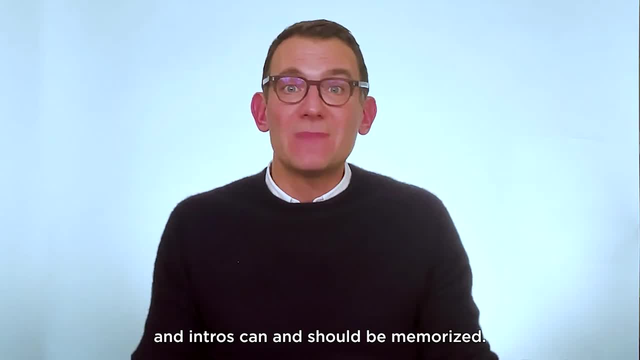 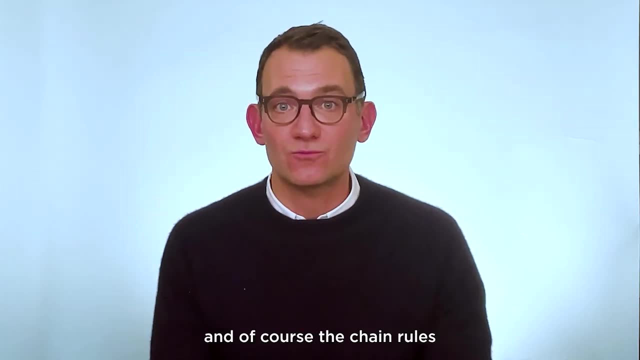 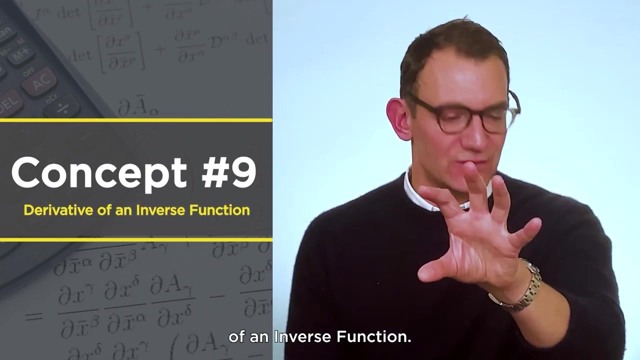 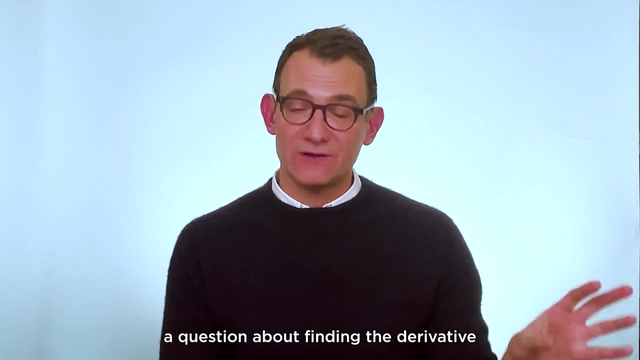 these derivatives and integrals can and should be memorized. Doing so will make it a ton easier to apply the product quotient and chain rules to these questions. Concept number nine: the derivative of an inverse function. The College Board will occasionally ask a question about finding the derivative of an inverse function, so you'll 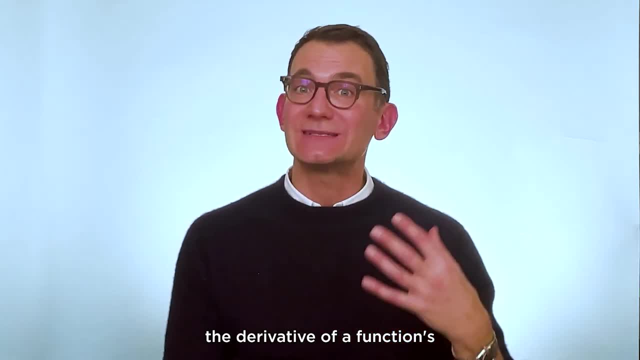 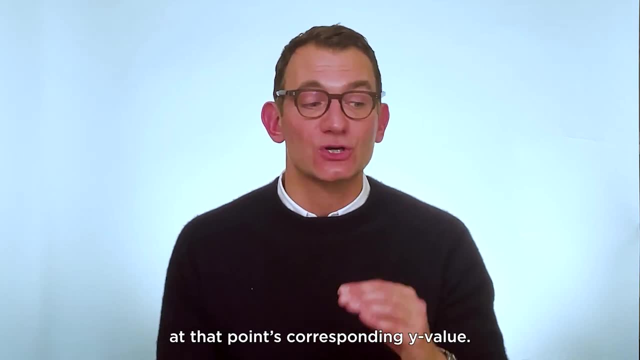 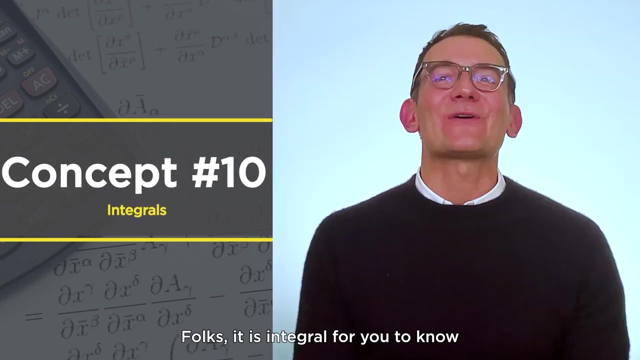 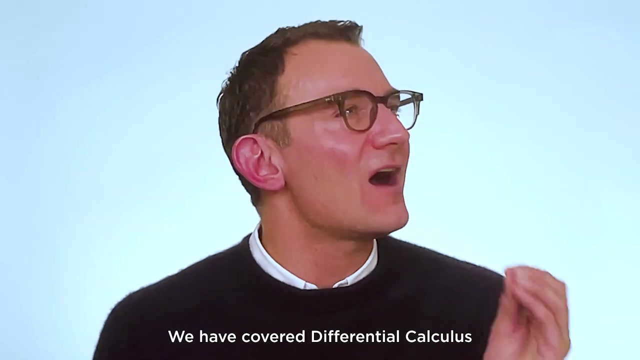 need to know how to find the derivative of the derivative of the inverse function. Concept: number ten: integrals themselves. Folks, it is integral for you to know about integrals. Bad jokes aside, my friends, so far- let's just look back- We have covered differential calculus. 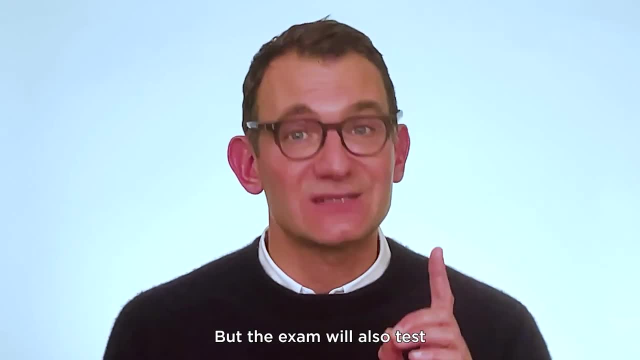 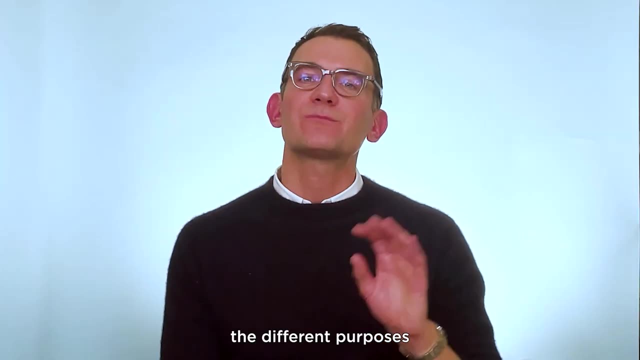 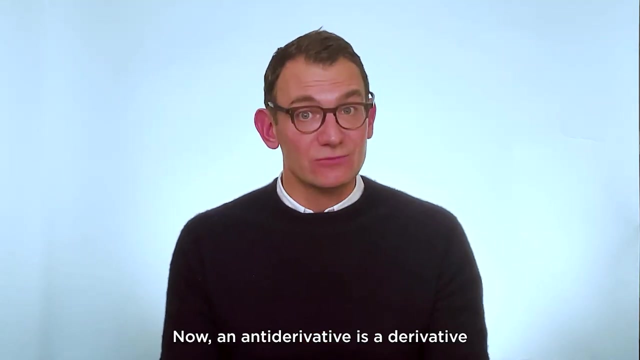 and what you need to know about the derivative. but the exam will also test you on the reverse- How to take an integral. You will need to understand the different purposes. an integral serves as the antiderivative. Now an antiderivative is a derivative in reverse. 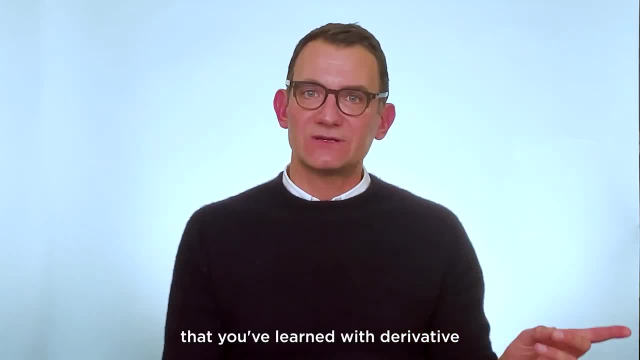 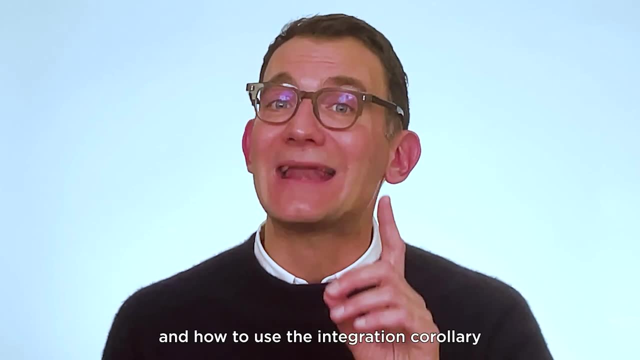 You should be able to apply the rules that you've learned with derivatives to integrals. For example, you should know how to reverse the power rule for antiderivatives and how to use the integration corollary of the chain rule called the U. 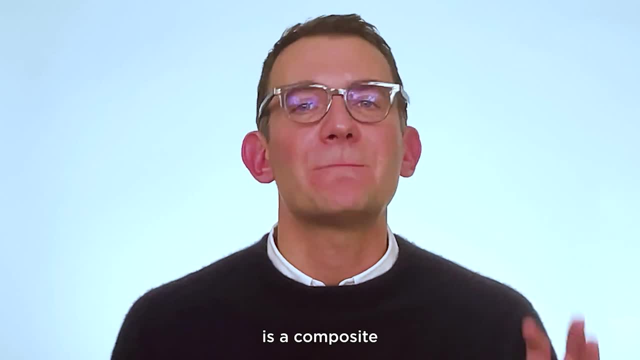 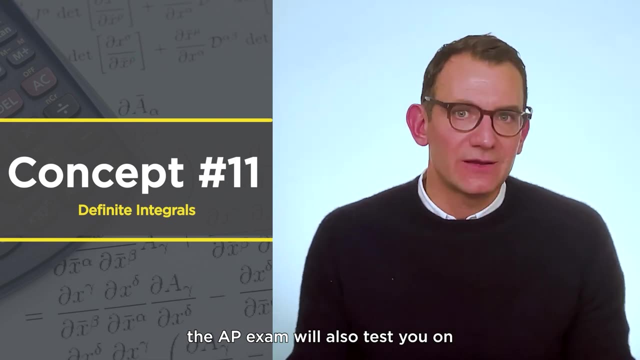 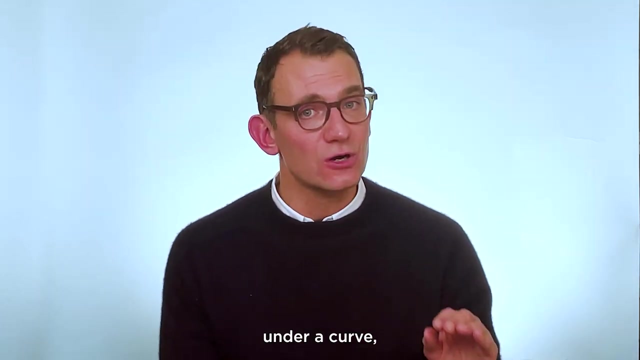 Substitution when the integrand is a composite function. Definite integrals Now. the AP exam will also test you on definite integrals, so you'll need to know how integration is used to find the area under a curve, including how to use rectangles. 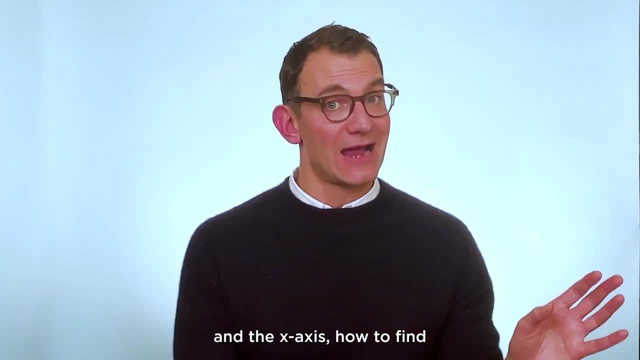 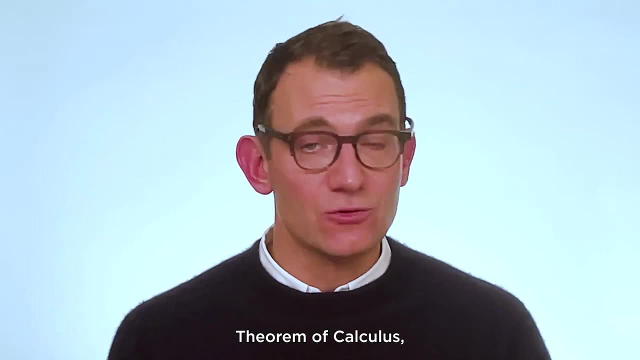 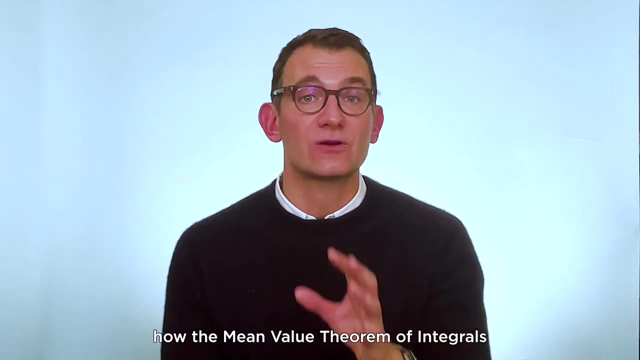 to approximate the area between the curve and the x-axis, how to find the Riemann sum and how to use 궁argand do after-affecting when the traverse rule is not confirmed. Next, you'll need to understand how the mean value theorem for integrals. 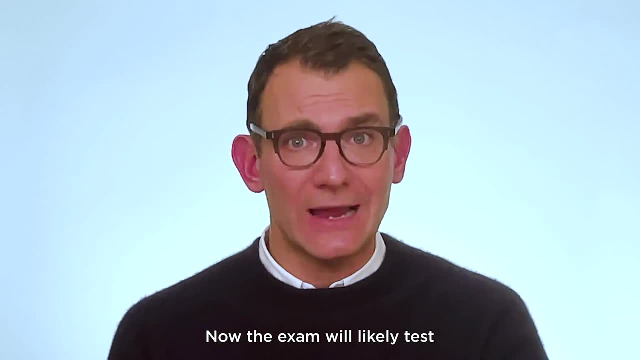 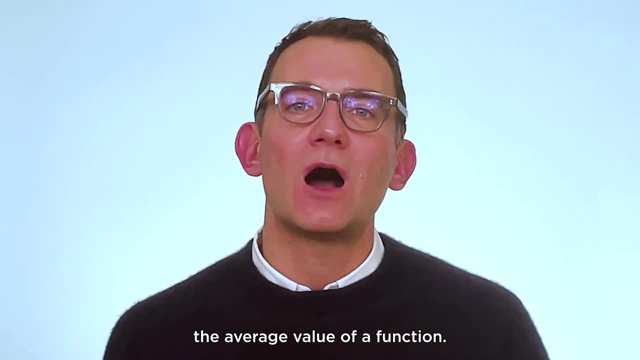 otherwise known as MVTI, applies to integrals. You'll need to know how the mean value theorem applies to integrals when the traverse rule is not considered. Next, you'll need to understand how the mean value theorem of integrals—otherwise known as. 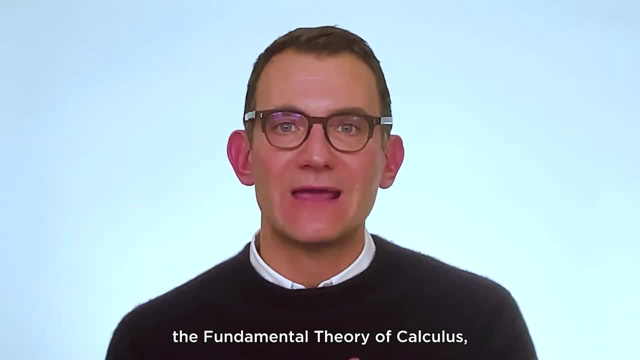 the acronym MVTI—applies to integrals. You'll need to know how the mean value theorem of integrals applies: bunchin intervals, specification of first, mu, communc, mu, p, etc. And you'll etc calculus. it is important to know that it has two parts of it. 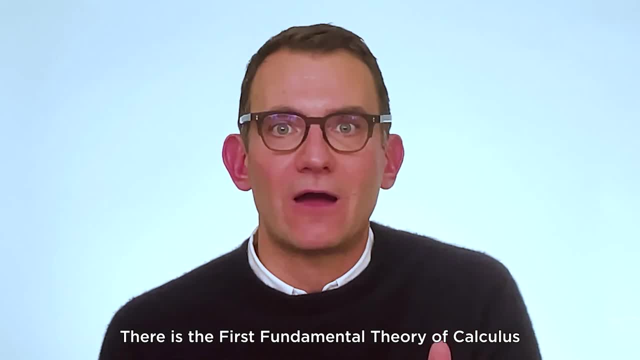 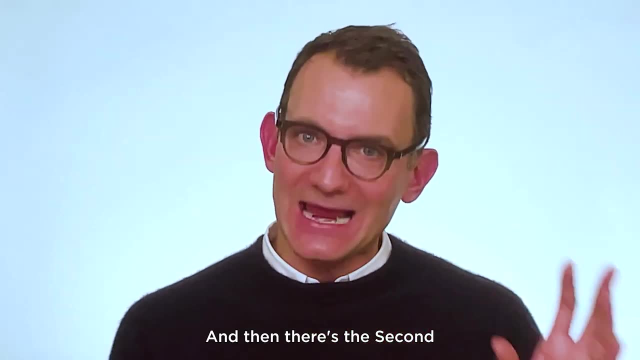 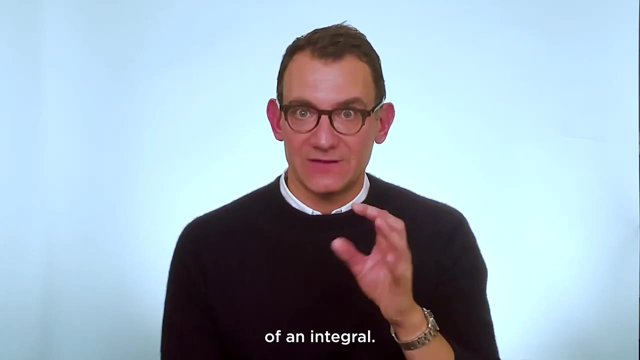 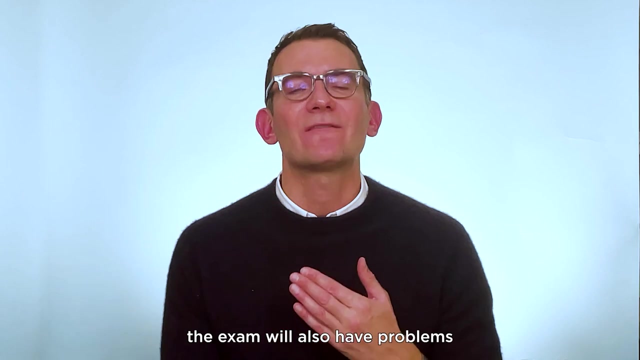 There is the first fundamental theory of calculus, used in evaluating definite integrals, and then there is the second fundamental theorem of calculus, which tells us how to find the derivative of an integral. Aim to understand both parts of this theorem And, lastly, the exam will also have problems that deal with accumulation functions. 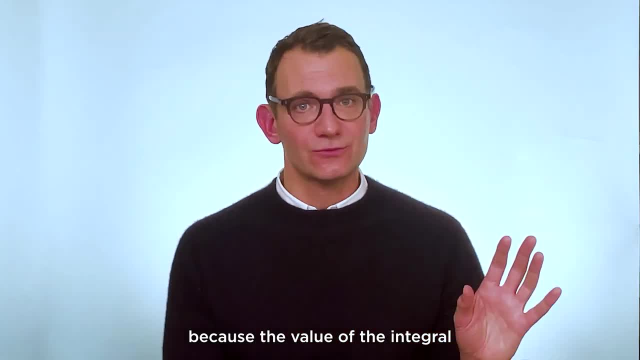 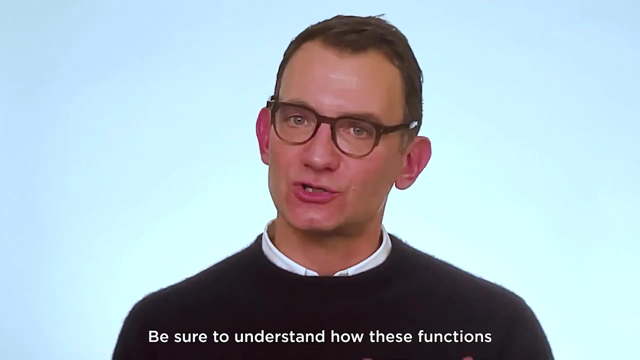 They're called accumulation functions because the value of the integral is the area under the curve from the constant to the value x. As x gets bigger, so does the area, hence it's called an accumulate. Be sure to understand how these functions work overall. 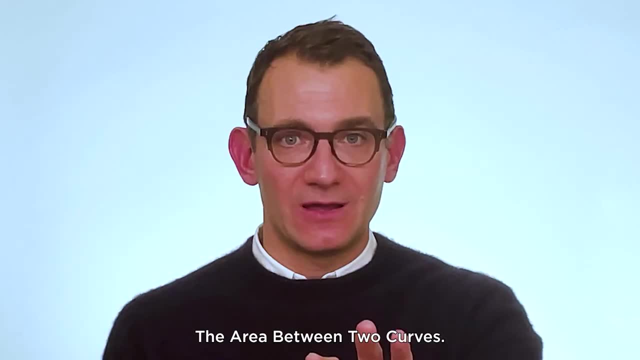 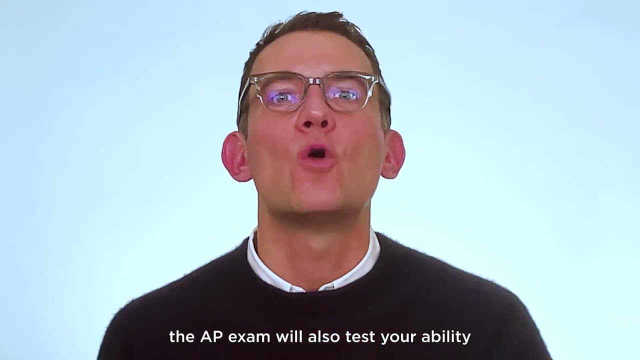 Concept 12. The area between two curves. In addition to the area between the two curves, the area between the two curves is the area between a curve and the x-axis. The AP exam will also test your ability to find the area between two curves. 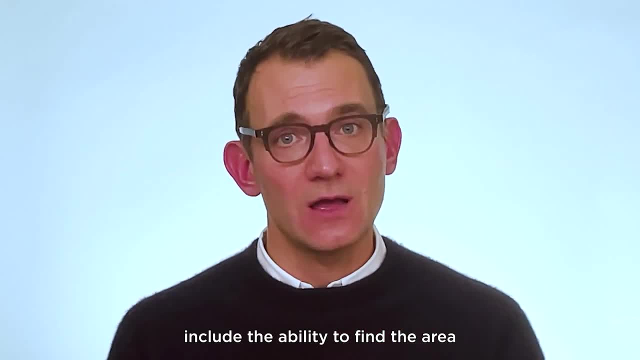 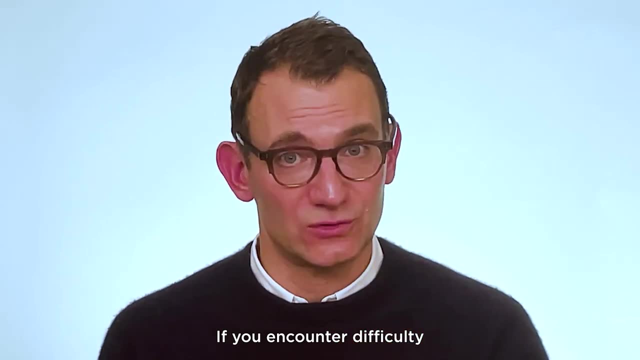 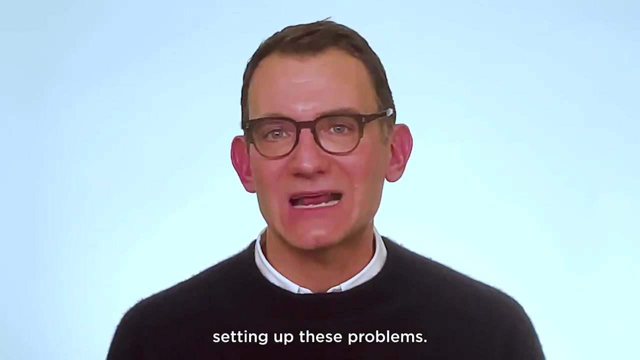 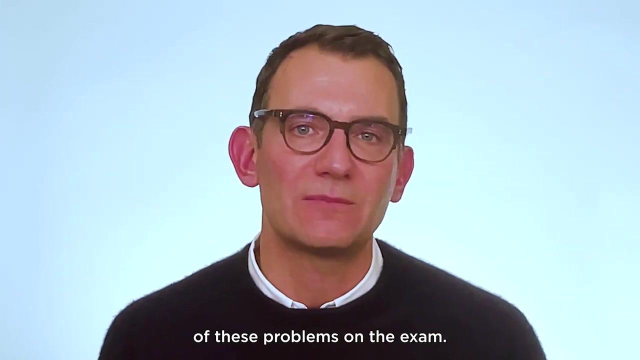 This will include the ability to find the area by slicing up the region both vertically and horizontally. If you encounter difficulty with this concept, know that you're not alone. Students often have trouble setting up these problems. Fortunately, the College Board asks relatively simple versions of these problems on the 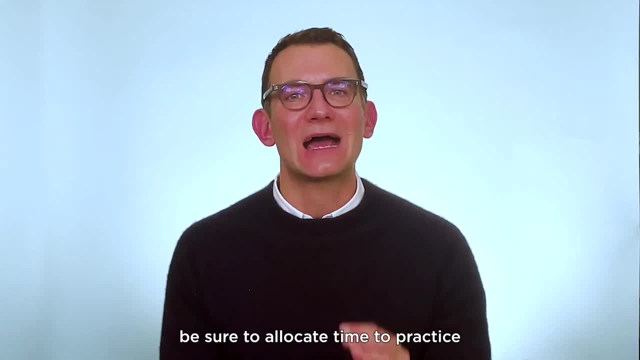 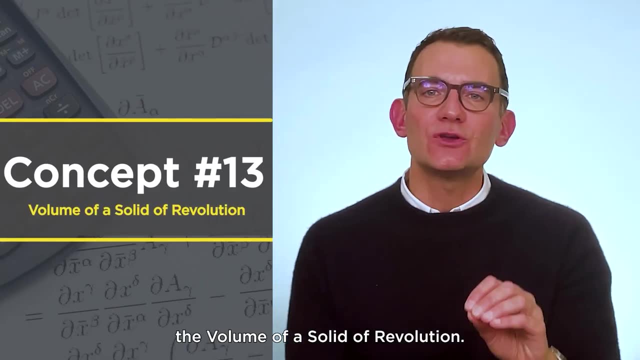 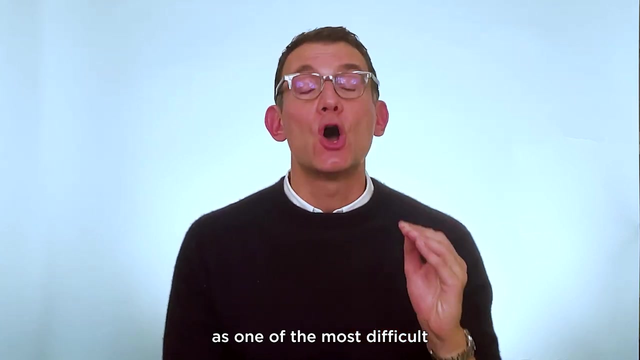 exam. That said, be sure to allocate time to practice this concept. Concept 13.. The volume of a solid of revolution. This concept is widely seen as one of the most difficult concepts on the exam and while there are always going to be volume questions on the exam, it's not always going to be a 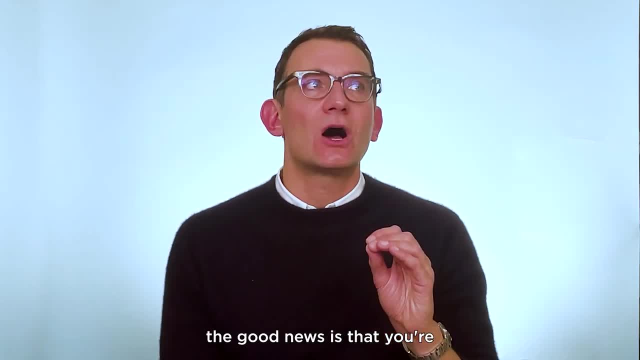 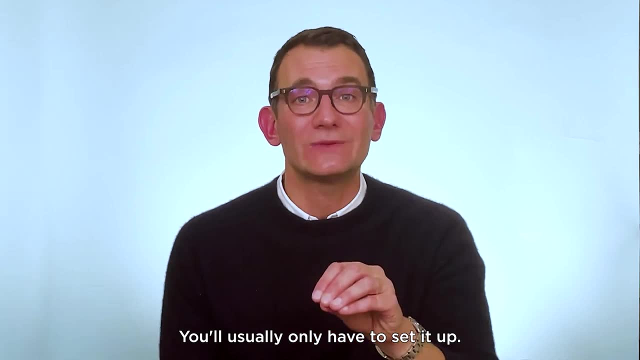 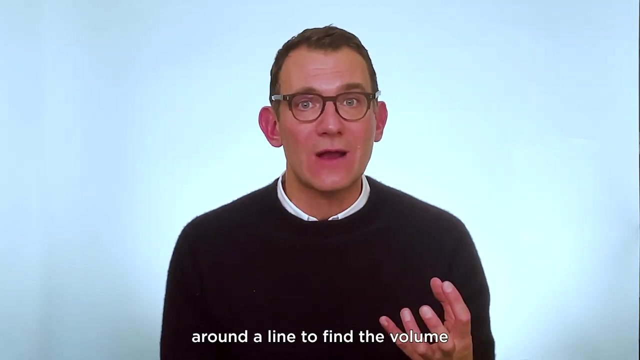 problem. The good news is that you're almost never- never- asked to evaluate the interval. You'll usually only have to set it up. You'll need to know how to take the region between two curves and rotate it around a line to find the volume of that particular region. 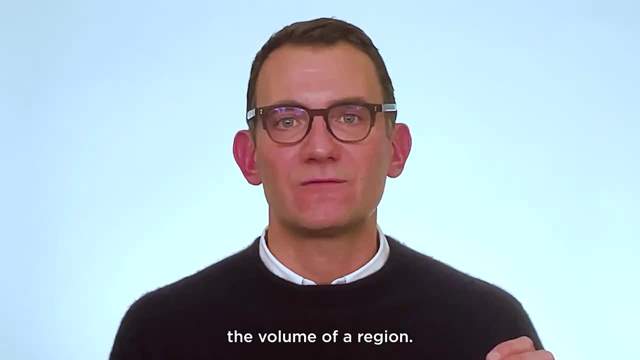 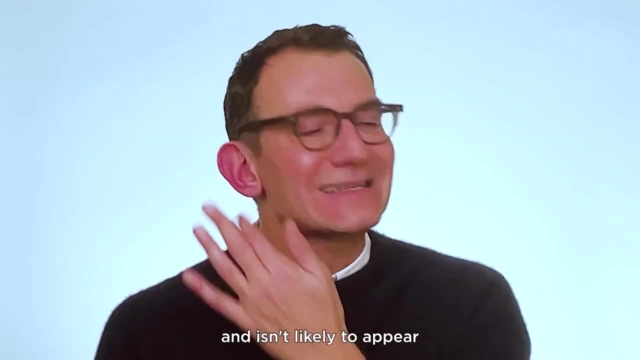 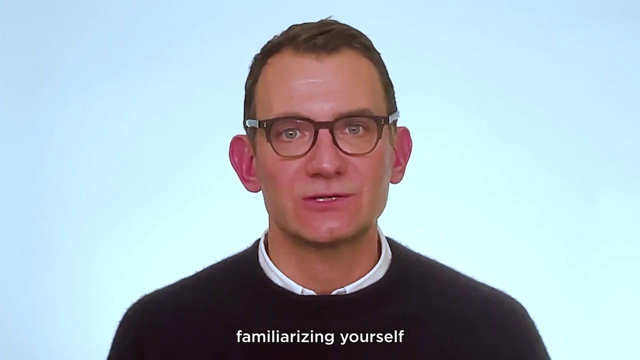 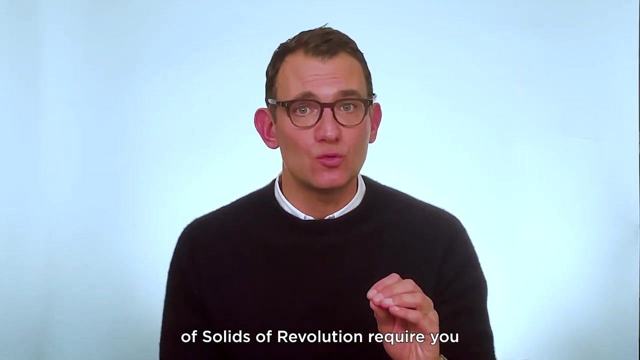 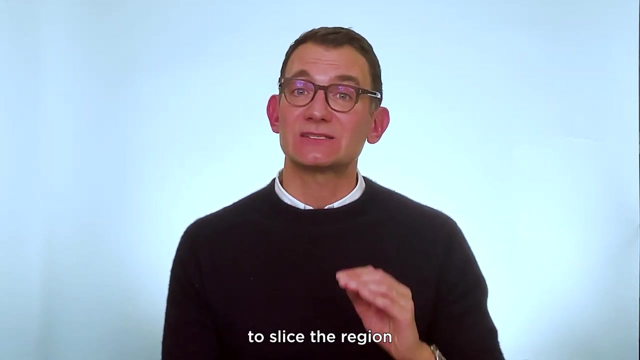 Friends, there are two methods to find the volume of a region: 1. The washer's method, 2. The cylindrical shell's method, 3. The ladder method, 4. The the slacer's method, 5.. 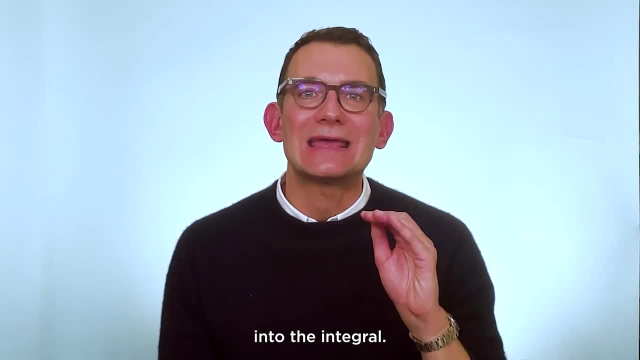 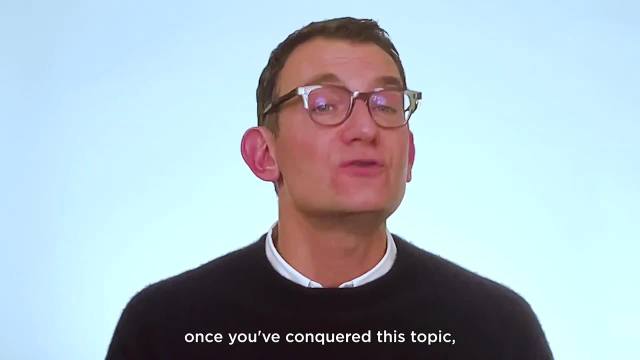 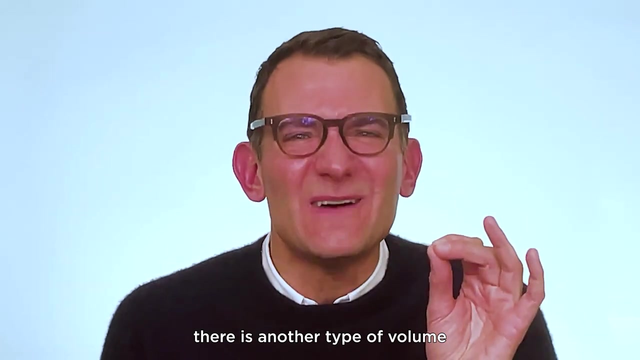 The j method 6. The ladder method 17. into the integral, Friends, with enough practice, finding the volumes will become far easier each time And, folks, once you've conquered this topic, you'll be ready for anything. That said, there is another type of volume that you need to be able to find. 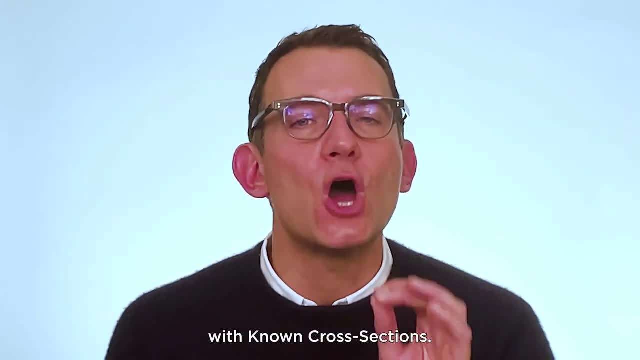 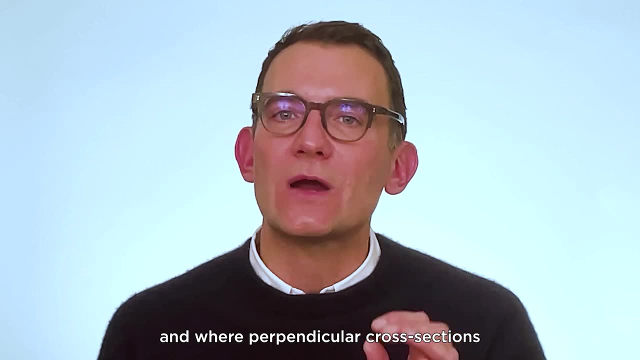 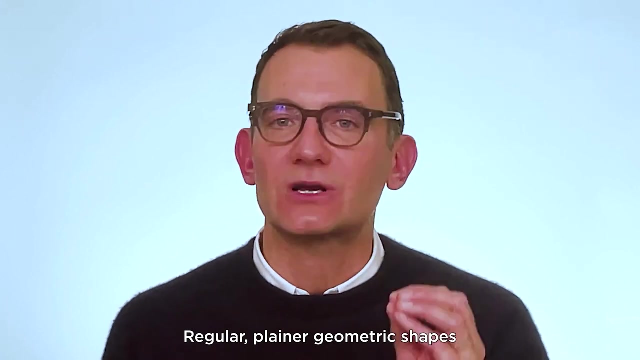 and it's known as the volume of solids with known cross-sections. Now, in this case, you will be given an object where you know the shape of the base and where perpendicular cross-sections are all the same—regular planar geometric shapes. You'll 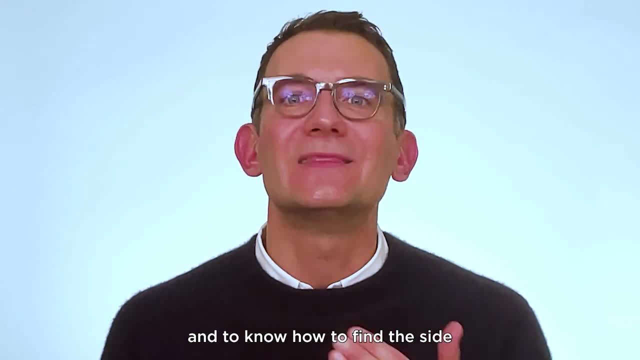 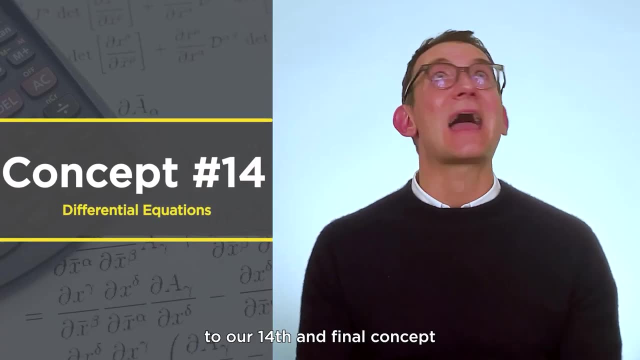 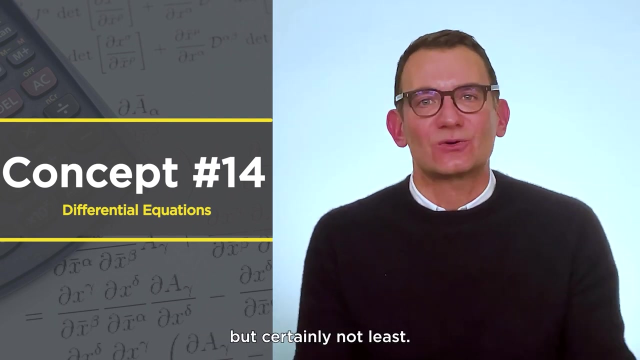 need to understand and know how to find the side of the cross-section in terms of y And friends. that leads us to our fourteenth and final concept on this calculus exam and it's differential equations. Now, this is, of course, last but certainly not least. You need to familiarize yourself with differential equations while you're at it. While you're at it, you need to familiarize yourself with differential equations while you're at it. While you're at it, you need to familiarize yourself with differential equations. 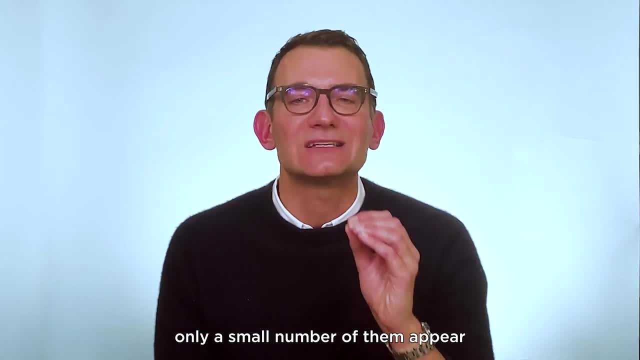 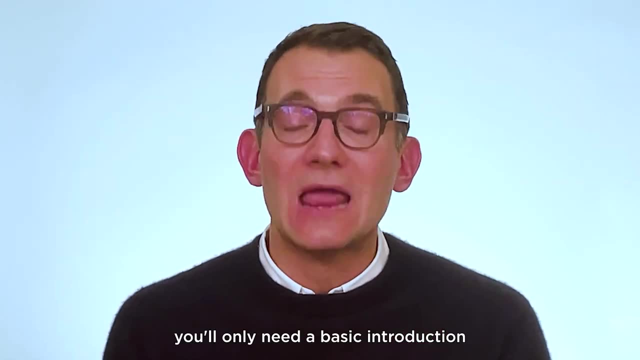 while you're at it, you need to familiarize yourself with differential equations. While there are many types of differential equations, only a small number of them appear on the Calculus A-B exam. As such, you'll only need a basic introduction to the topic on test day. first, You'll need to 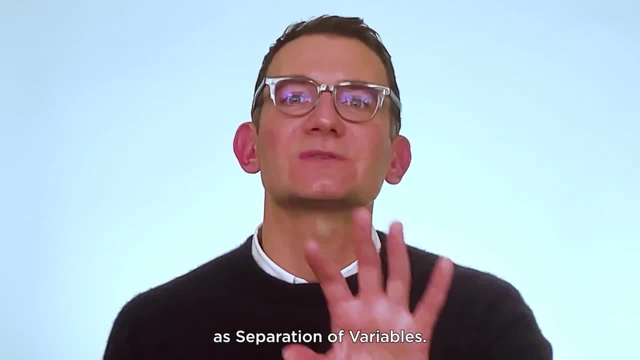 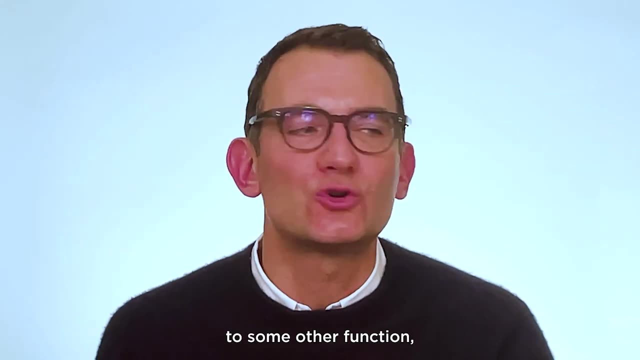 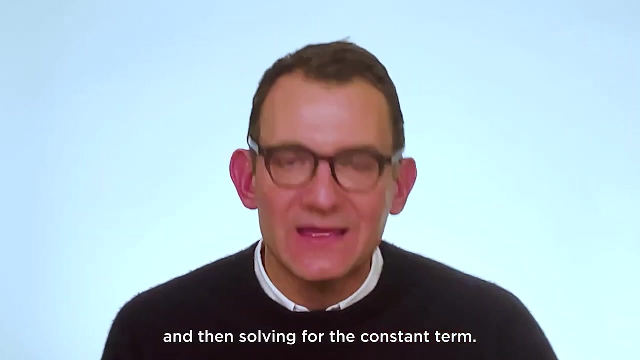 understand the method known as separation of variables. If given an equation in which the derivative of a function is equal to some other function, you should be able to determine the original function by integrating the derivative of a function into the derivative of a function. By integrating both sides of the equation, you'll solve the constant term.